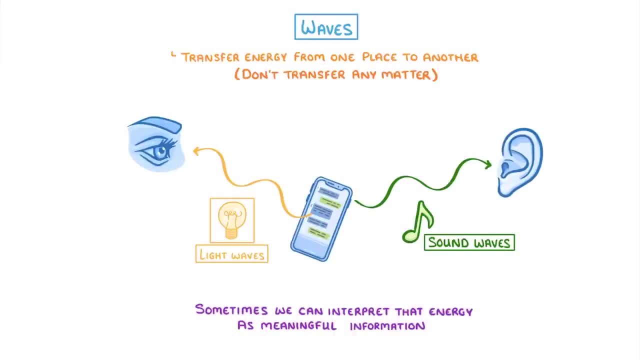 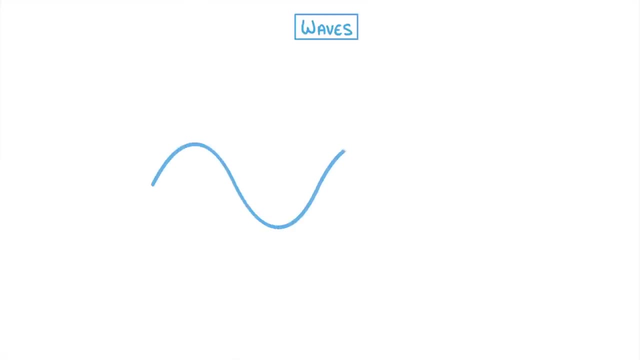 brain is able to build up images and tunes from the light and sound that it receives. To travel from one place to another, the waves vibrate or oscillate, as we can see in this displacement distance graph. The distance is how far the wave has travelled from the starting point, while the displacement 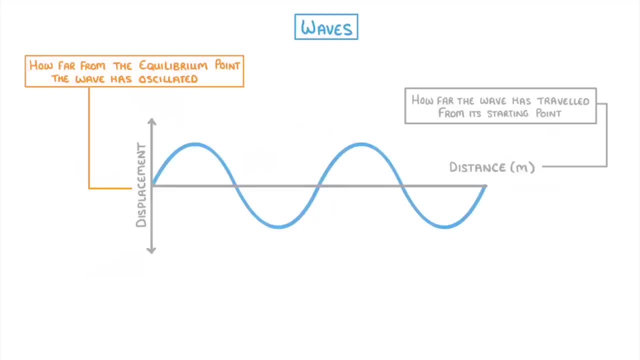 is how far from the equilibrium point the wave has oscillated, How far it's gone up or down. The maximum displacement is known as the amplitude amplitude, while the distance of one entire oscillation is called the wavelength. So that could be from equilibrium up down and back up. 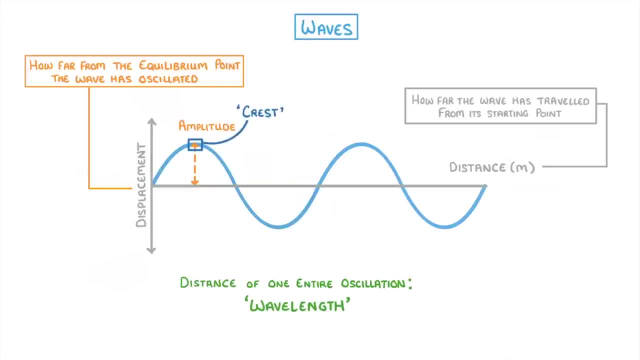 Or it could be from the very top of a wave, which we call the crest down, and back up to the next crest. It just has to be one entire oscillation And the opposite of the crest is called the trough. Now sometimes you might see a displacement time graph instead, which looks pretty much. 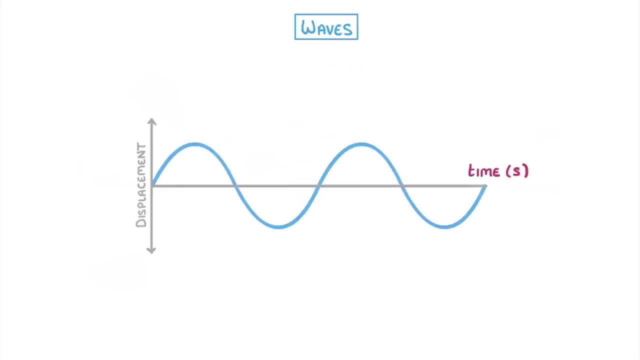 the same, but because we have time on the x-axis instead of distance, the length of one complete oscillation would be the time period instead of the wavelength, And the time period is just the time it takes for one complete oscillation. The benefit of knowing the time period is that we can then 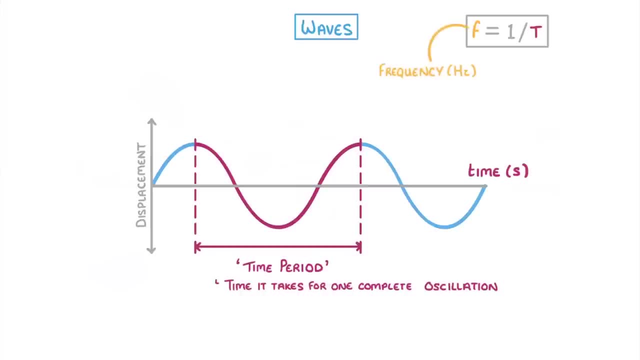 use the time period to calculate the length of the oscillation. Let's use this equation here to work out frequency, which is measured in hertz and is the number of complete oscillations per second. To see how it works, imagine that each oscillation takes 0.5 seconds. 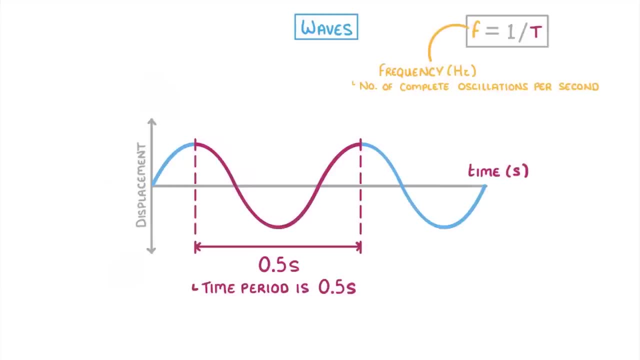 Or in other words, the time period is 0.5 seconds. This means that there must be a total of two oscillations per second. So the frequency of each oscillation is 0.5 seconds And the frequency is 2, which is what we'd get if we did 1 divided by the time period. 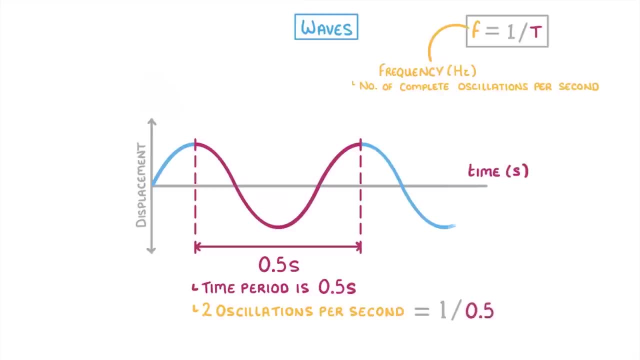 of 0.5.. We can also use the equation the other way round. so time period equals 1 over frequency. So if we were told that the frequency of a wave was 4 hertz, which means 4 oscillations per second, then to find the time period which is 0.5 seconds, we'd have to find the. 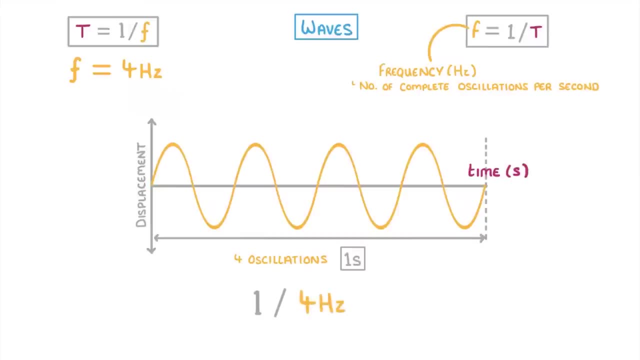 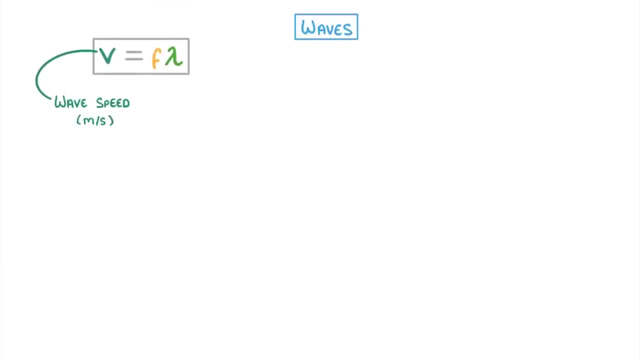 length of the oscillation. So let's just do 1 divided by 4, which tells us that each oscillation must be 0.25 seconds. The next equation to know is that we can find the speed of the wave, so the wave speed. 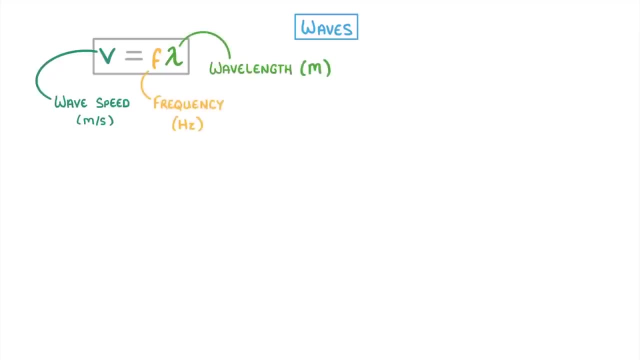 by multiplying the wavelength by the frequency. So basically, we multiply how long each wavelength is by how many there are per second. So by multiplying how long each wavelength is by how many there are per second, we get 1.25 seconds, and that will give us the total distance they travel per second. 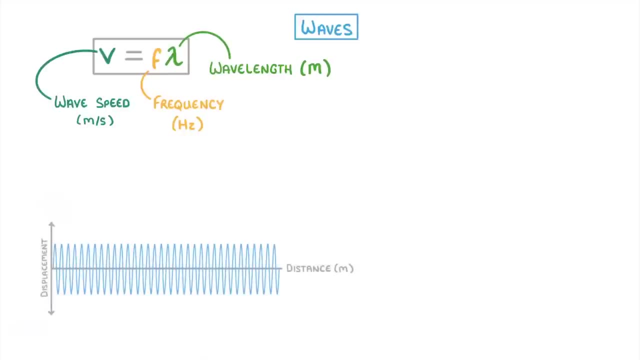 To see how this works, let's imagine we had a sound wave that had a frequency of 400 Hz and a wavelength of 70 cm. What is its wave speed? Well, in this case, all we'd have to do is convert the 70 cm to 0.7 m. 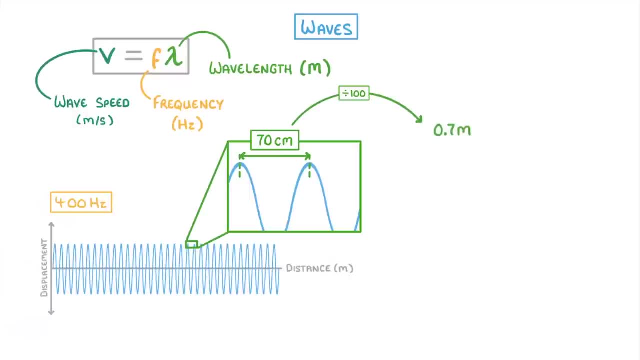 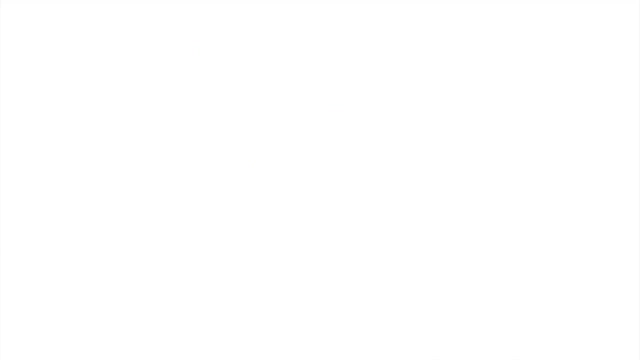 because we always want our wavelength in metres and then multiply it by their frequency of 400 Hz, which gives us 280 m per second as our wave speed. The last thing we need to look at are the differences between transverse and longitudinal waves. In transverse waves, the oscillations are perpendicular to the direction of energy transfer. 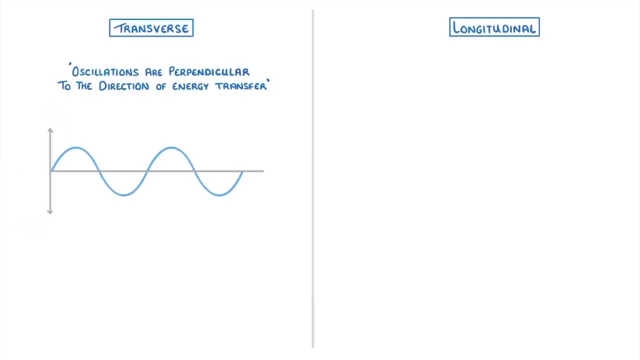 or the direction of the wave. The oscillations are perpendicular to the direction in which the wave is moving, which is why, on our drawing, the vibrations are going up and down whilst the overall wave is travelling from left to right. Most waves we can think of are transverse. 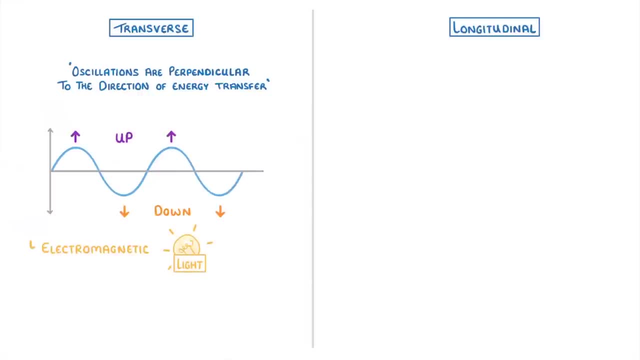 including all electromagnetic waves like light and radio waves, ripples and waves in water and the waves of strings like on a guitar. Longitudinal waves, on the other hand, have oscillations that are parallel to the direction of energy transfer. This one's a bit trickier to get your head around.